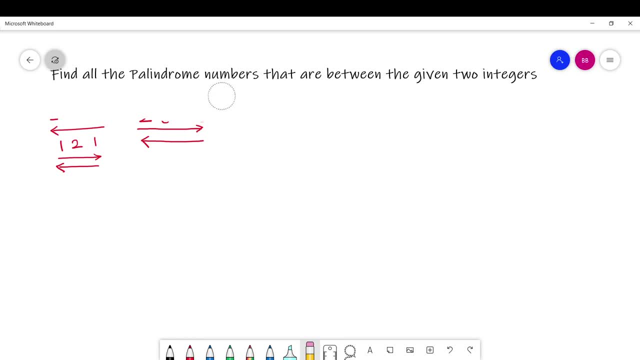 So, before we address the question of finding out the various palindrome numbers between two given integers, we will try to find whether the given integer is palindrome or not, Which means if user is going to give an input. which means if user is going to give an input. 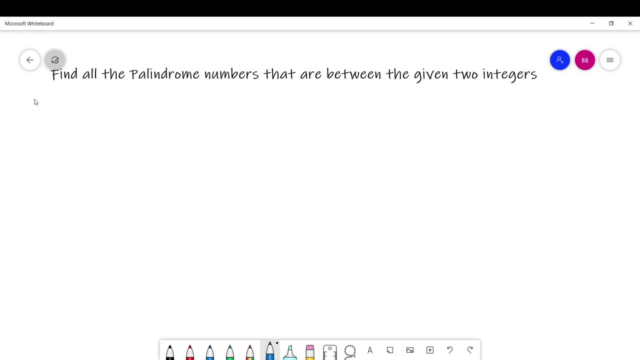 which means if user is going to give an input, that number would be read as input and we will find whether that given input number is palindrome or not. So we will write an algorithm for this That is read: num. temp equals num, which means the num is the one which is. 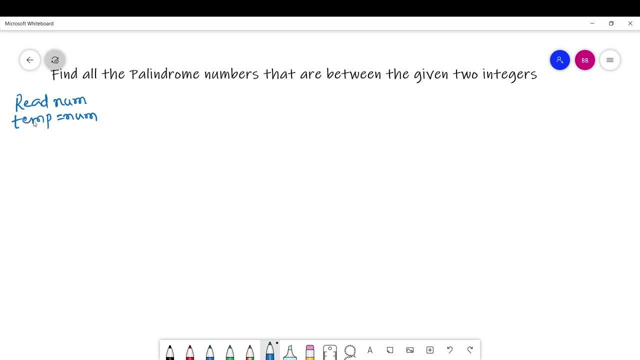 read from the user and we are attaching it to a temp and we will have to find the reverse of it. also why we will have to find the rewards, because the actual number and the reverse of that number should be equal, so that those would be a palindrome that is zero while, which means we'll have to find each and every. 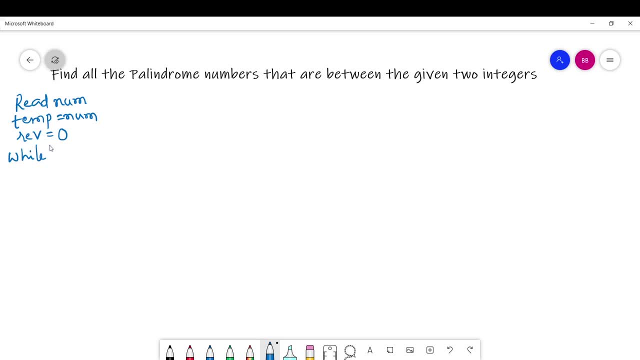 digit. we will have to check each and every digit, so for which we are going to write a logic where we are going to introduce a loop and this loop is going to calculate the new given number is palindrome or not. so the remain, we are going to use a remainder. remainder is temp star 10. then 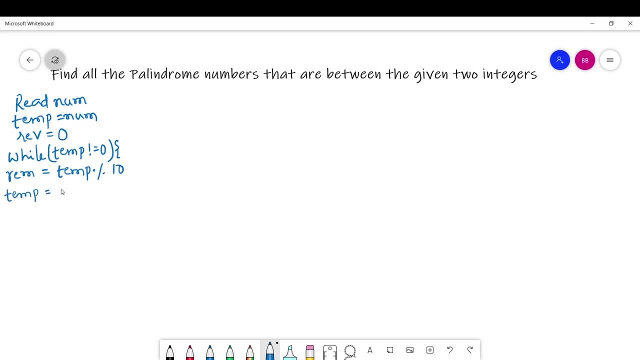 temp will calculate the new temp, and new temp would be temp slash 10. and then we will find the rewards. rewards is equals to rewards star, 10 plus remainder. and this, these are the three statements we kept in the loop after n number of iterations. it all depends on how many number of digits are there in the loop. so we have 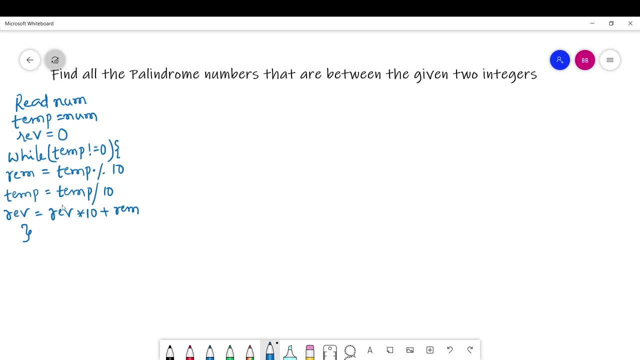 there in the given number. so, depending upon that, this takes number of iterations. so after all the iterations, reverse would be calculated. so now, after the reverse is calculated and the while loop is broken, we will check whether the given number is equals to the reverse of the number. 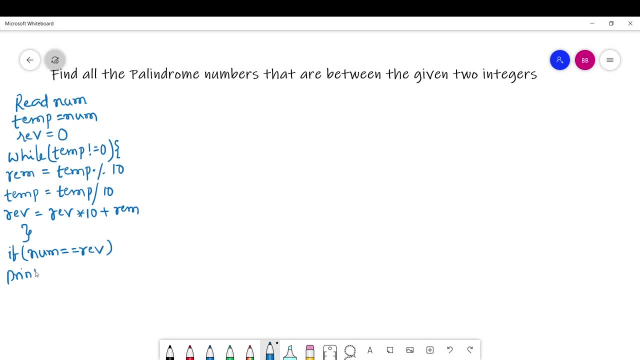 if it is equals, then we will print. the given number is palindrome or not. okay, this is what the logic is, so for which what we do is: we will take an example. we take an example: the given number is 121, so this 121 is assigned it. 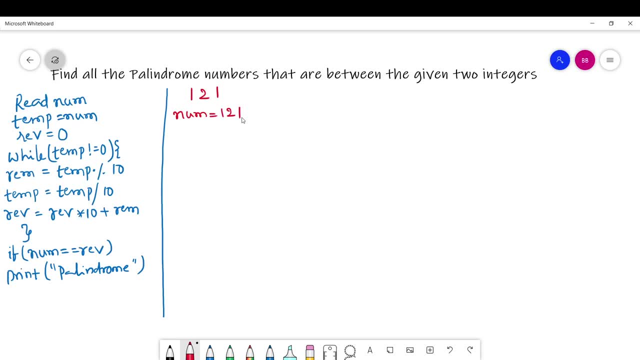 to number. so because when the user number is given that number is stored in 121, then that same number is stored in temp. the temp would contain 121. so temp is equals to number and number having 121. and that went when 20 is aside to temp. 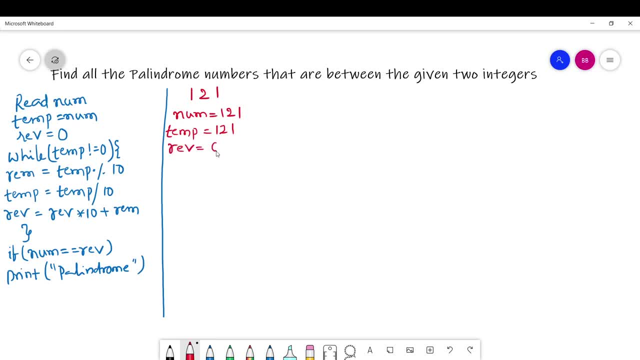 then rewards is equals to 0, while temp is not equal to 0. what is the value of temp? 121 is not equal to 0. is it not equal to 0? yes, so because of which we start with the first iteration, for in the first iteration, remain equals to 121. 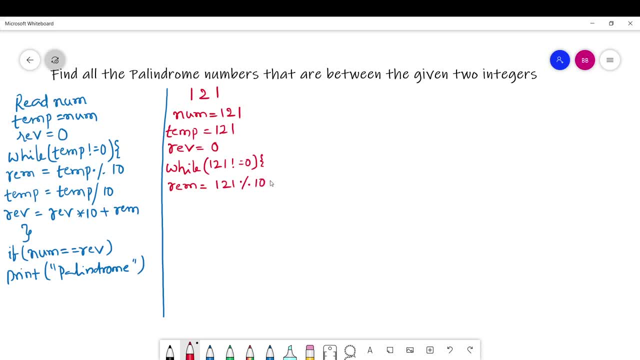 percent, 10 and 121 percent and is equals to E to 1, and temp equals to temp slash 10. what is the value of temp? it is 121, 121 divided by 10, which is equals to 12. then these are the statements. then we have to calculate the reverse. reverse is equals. 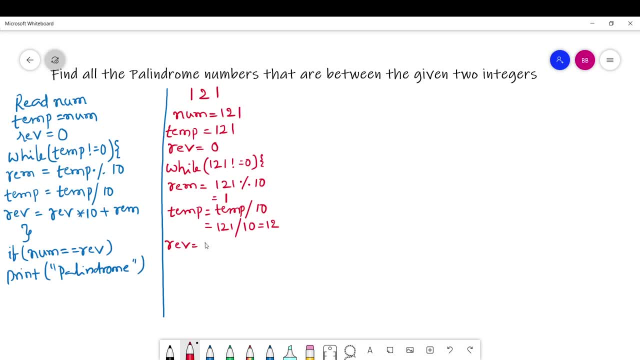 to what is the value of reverse? the presently value of reverse is 0, 0 into 10 plus what is the value of remainder 1, which is equals to 1? so this is the first iteration. this is first iteration. let us see the second iteration, the next iteration. in the next iteration we are going to carry the 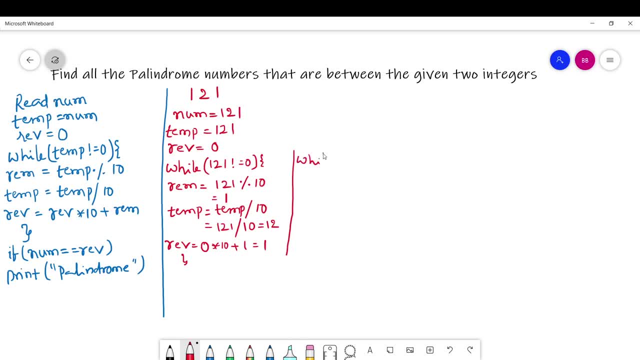 value of temp as 12. so, while 12 is not equal to 0, is it true? yes, because it is true. it enters into the loop and remainder is equals to 12 percent 10, which is equals to 12 percent 10 is remainder is 2. so temp is equals to 12 slash 10, which is equals to 1. then, 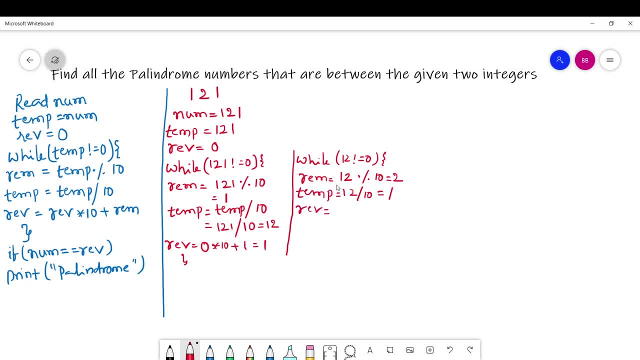 reverse is equals to what is the value of previous reverse. so we have already one. one starts 10 plus remainder. what is remainder? 2, which is equals to 1, into 10. 10 plus 2, that is 12. so now we have calculate the reverse. in the 3rd iteration you can address the arsenal. 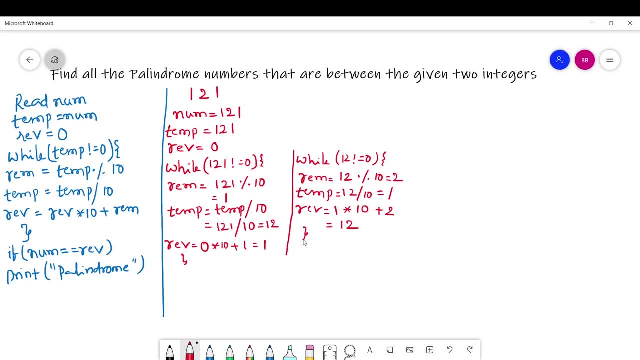 because second iteration is done and temp is not equal to 0. so we will enter into 3rd iteration. in the 3rd iteration is in the emperor will enter into. third iteration is infinite constraint. this As let us name, advanced veioz. so if the p should be 0, Eического the bracket is this, we'll do the 3rd iteration. if this insert would be 0, TEMPS equal to 1 and temp is equal to 0, 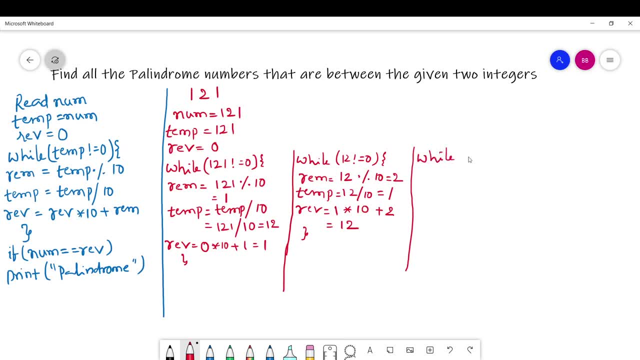 iteration. Our new value of temp is 1.. 1 is not equal to 0, which is true, So it enters into the loop. Remainder is equals to 1 slash 10, which is equals to 1.. Then temp is equals to 1 slash 10. 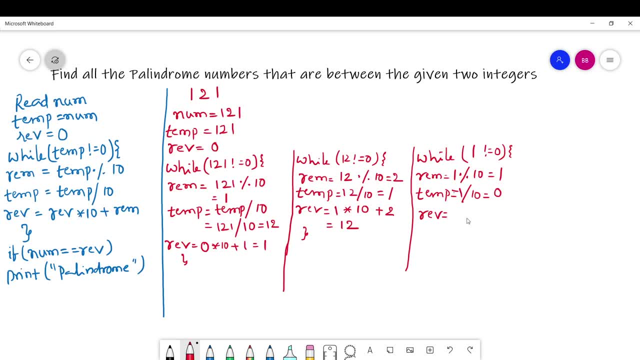 which is equals to 0.. Reverse is equals to old, reverse is 12.. 12 into 10 plus the remainder is 1.. So this is 120 plus 1, which is equals to 121.. So this is computed. The next iteration let us. 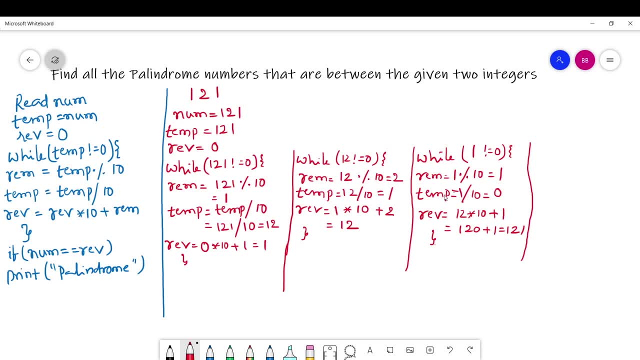 see whether we will be able to pass through the next iteration or not. What is the value of new temp, while 0 is not equal to 0, which is false. So after we got the loop broken, which is left over, we have to compare with the reverse. If, what is the value of num 121.. 121 is equals to the reverse rev. What? 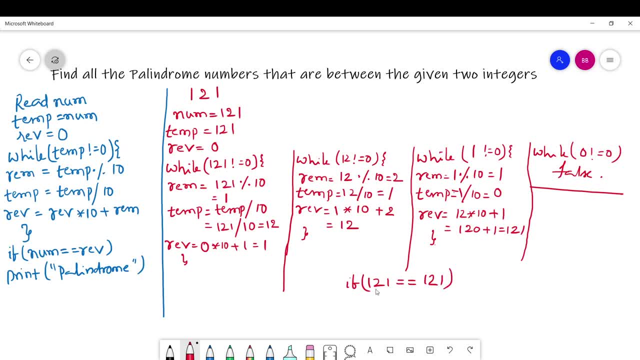 is the value of rev 121. Because both are same, 121 is equal to 0. So this is false. So after we got the loop broken, which is left over, we have to compare with the reverse. So this is 121.. 121 is equals to 121.. We will print it as a palindrome, So this: 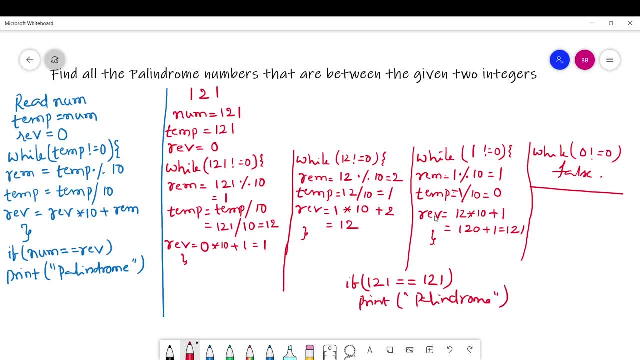 is the logic for finding out whether the given number is palindrome or not. But now our question is to find the logic or to find all the palindrome numbers that are between the two given numbers. So when we have to find the logic for given two integers, we are going to 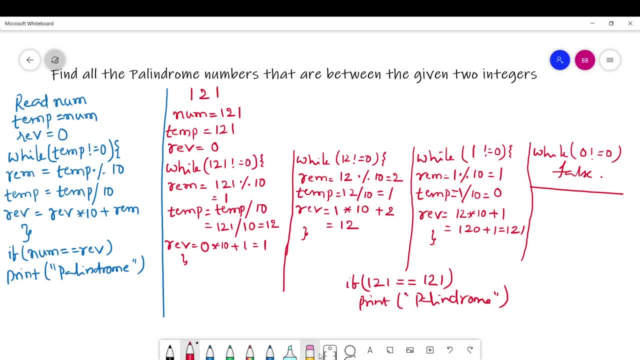 change the logic a bit. So how do we change this logic? Let us see. I will clear this So that we will just by the side of the same logic. we will write the logic for finding out the palindrome numbers that that are between two given. 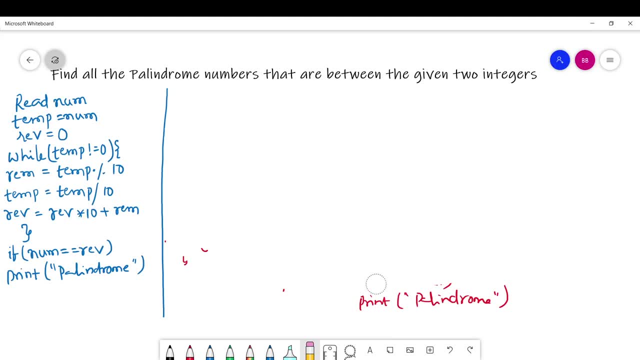 given integers. we will clear the screen here. okay, we will write the logic here. what is the logic? because, given two integers, so obviously it means that we will write. we will read two integers, that is read first number and second number. then, once we read the first number, the second number, which means 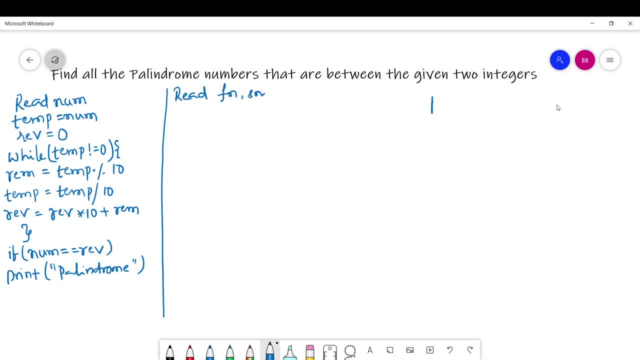 this is the first number and this is the second number. between these two numbers, between these two numbers, this is a first number and this is a second number. between these two numbers, there are n number of numbers among which there might be few palindromes. I mean, unless we check, we can't say. but there is a. 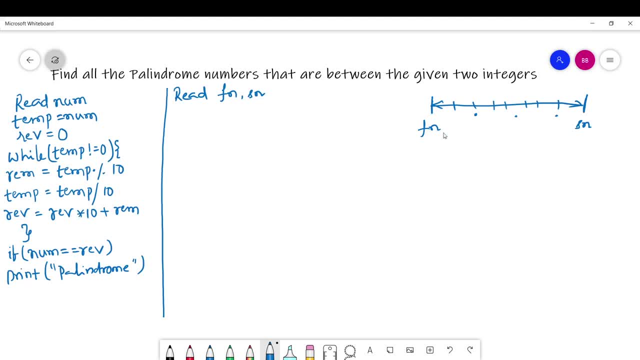 possibility of having the palindrome numbers between the first number and the second number, that is, between two given integers. we have to find them, so the first number becomes a lower bound and second number becomes the upper bound, which means we start with finding out the palindrome with the first number and keep on incrementing by one and until we 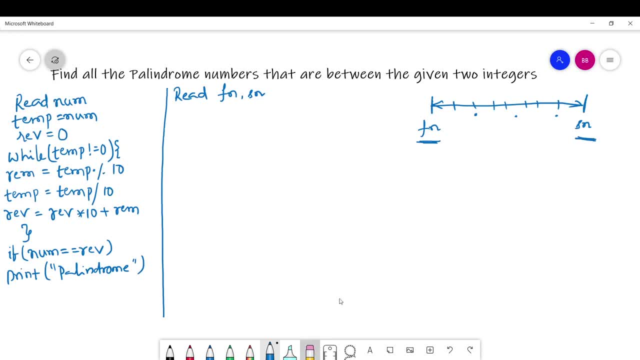 reach the second number that is upper bound. so we will go through with this particular logic and we will see how many numbers that we get. okay, so now, because now. so anyways, I know how many letters are necessary, because now we are going to calculate for the first given number. so numb is first number. we 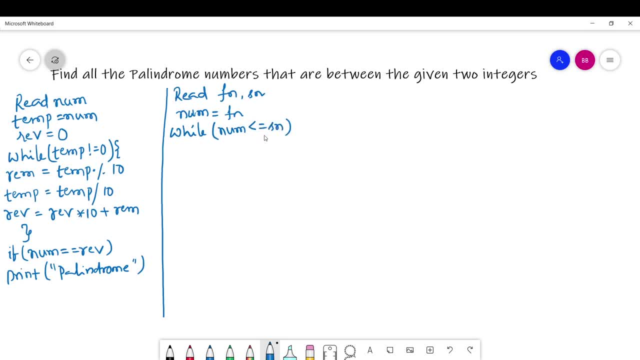 are going to add another loop, for number is less than or equals to second number. why this number is less than, equals the second number. what is that? number first will reach the last number, that is, the second integer or the second number, so that becomes the upper bound. so, and from the lower bound till the upper bound. we have to check, we have to keep. 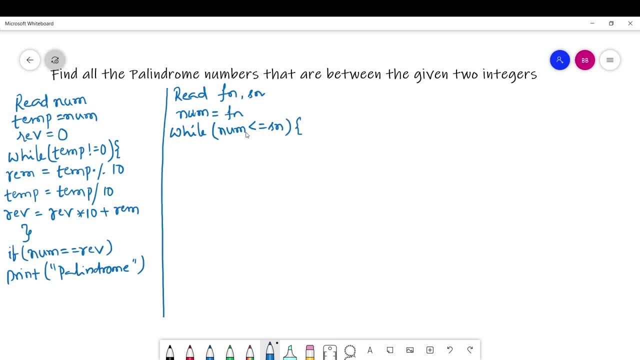 on incrementing. that is why this specific condition: the number is less than or equal to second number, then obviously we are going to continue the same logic: temp is equals to num, then reverse is equals to 0 and, as usual, while temp is not equal to 0, remainder is equals to temp. 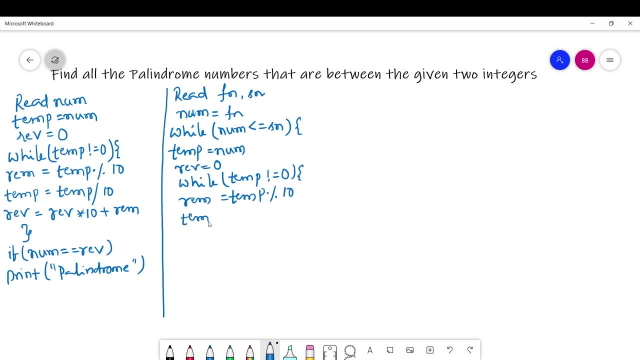 percent 10. temp is equals to temp slash 10, then reverts is equals to reverse star 10. we have to compute the reverse of the given number right, then the inner loop is closed. if number is equals to reverse of that same number, then we have to print the palindrome that is number. 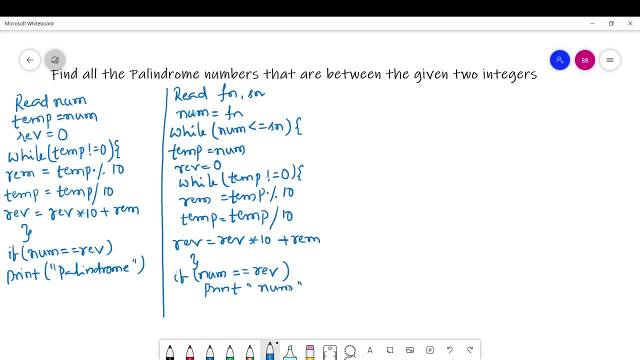 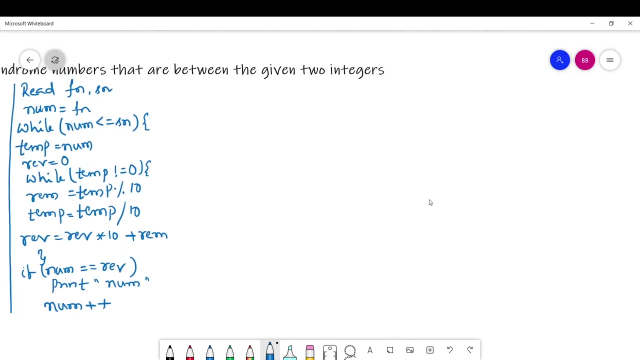 okay, this is what the logic. but because we have to keep on incrementing until the upper bound, we are going to add num. we are going to add another instruction, which is num plus plus. okay, this is for the logic. this logic is for finding out the palindromes between two given integers. we will adjust this. 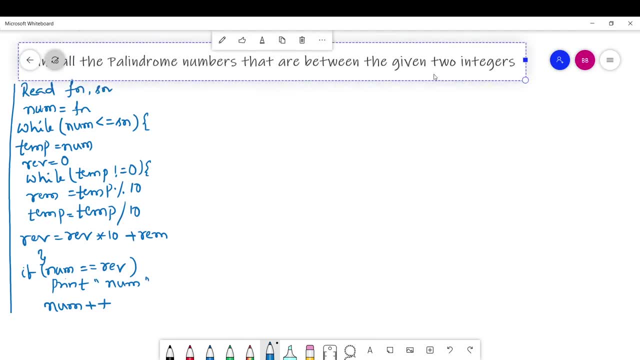 okay, so we will see this now. having this, we will try to evaluate with a few examples. let us say we are asked to find the palindromes between two numbers that are 10 and 25. so obviously this becomes first number and this becomes second number. so according to the logic, 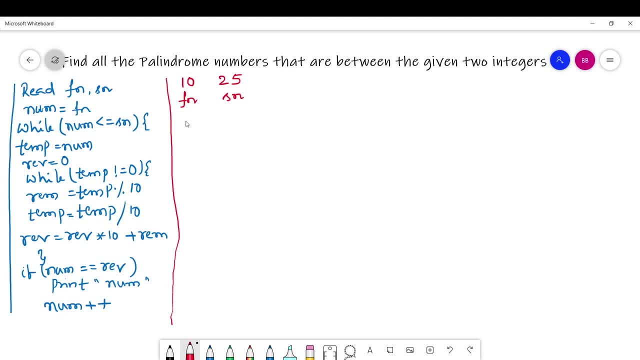 the first number is assigned to num, so num equals to first number, that is 10, while number is 10. 10 is less than or equals to second, which is second number, that is 25.. if it is 25, then temp is equals to num, that is, temp will also contain the value 10.. 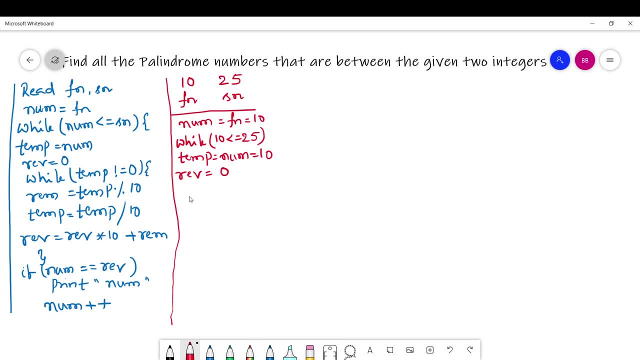 as usual, reverse is going to be 0.. so, while we are going to start another loop, while num, while temp, is not equal to zero, which means the present value, which is 10, is not equal to zero. yes, it is not equal to zero. because it is not equal to zero, it enters into the first. 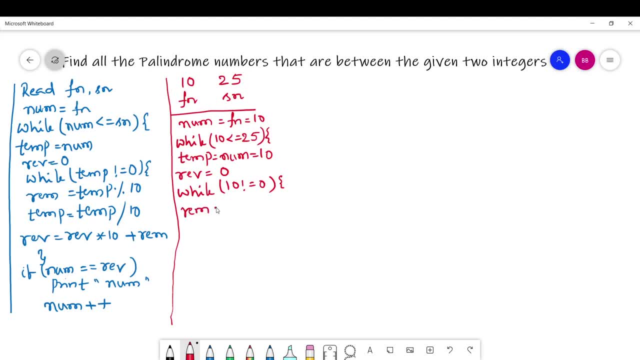 iteration. so as part of that we will calculate the remainder. remainder is: what is the value of temp? temp 10, and then 10 percent 10. 10 percent 10 is zero, then temp equals to temp slash 10, that is, 10 slash 10, which is equals to one, and then reverts is equals to reverts. what is? 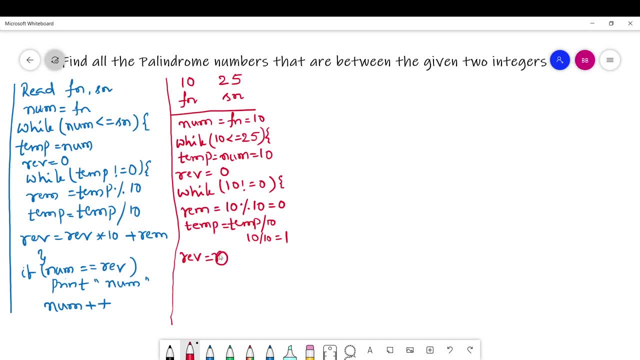 the value of reverse here: 0. this is 0. star 10 plus remainder is 0, which is equals to entire value is 0. so this is the first iteration. what about the second iteration? let us see whether it can reach the second iteration or not. so 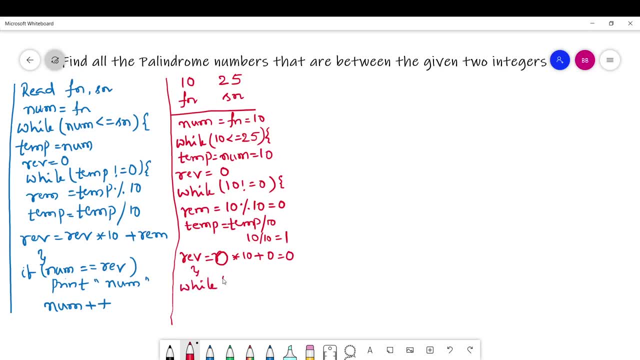 the. we are going to carry with the value temp value as 1. 1 is not equal to 0, which is true because it is true remainder is equals to 1 percent. 10, which is 1. temp is equals to 1 slash. 10, which is 1 temp is equals to 1 slash. 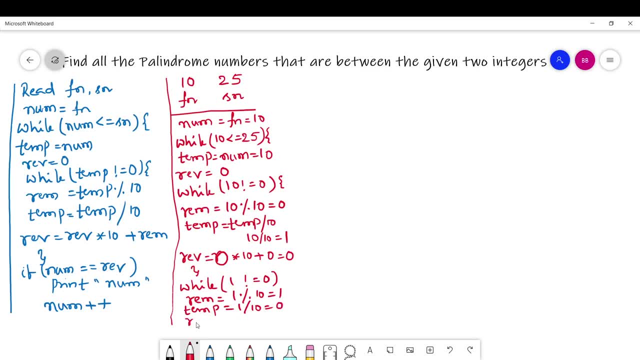 10, which is 1, temp is equals to 1, slash 10, that is 0, and reverse is equals to earlier. reverse is 0, 0 star 10 plus remainder, that is 1, which is equals to 1. so this is the second iteration. let us 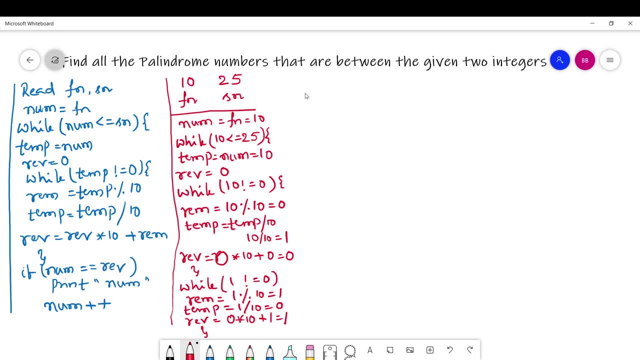 see if the first third iteration would be completed or not. so in the third iteration we are going to have a. the value while temp value is 0 is 0 plus 아니에요, cookie set to 0, which becomes false because it files a state. 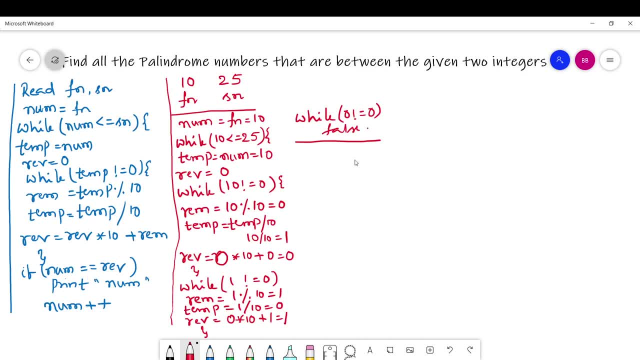 function is 기�ész to class. Once that is the case, let us want to check if and when we have to alter this. set in the order of 0 from the digit plus number, value 10. the resulting function in here is 10, so it is the Sol e. the function in here is equal to 0. we want. 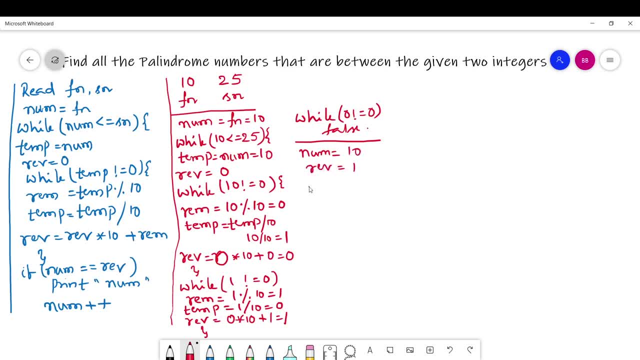 o not equal to 1. so the first iteration will be equal to 10, which is FALSE. does it mean? is it in this way we need to? This is also called the Schumacher redemption. the 3 Jedi loop is broken. once the loop is broken, what we need to do? because we have to check whether number, that is, number- is 10, whereas reverse. we have to do this because most numbers is not values and reverse is 1. and when I do this, I can see it is known that inside these scores will. Sorry, because we have to change that. 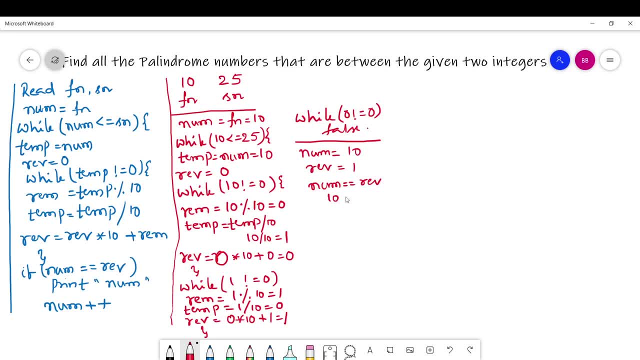 equals. to reverse, that is, 10 is equals to 1. this becomes false. so this is not going to be a palindrome. 10 is not a palindrome. so what we do? we are going to increase the value, so because of which num++, num++ becomes 11, so this 11 is: 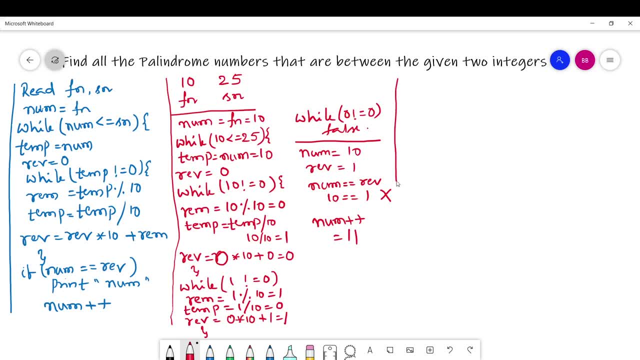 going to be the next one, which is which we are going to check whether it is palindrome or not. so we are going to once again start with the loop. so when, once 11 is given, we are going to check with this. while 11 is less than or. 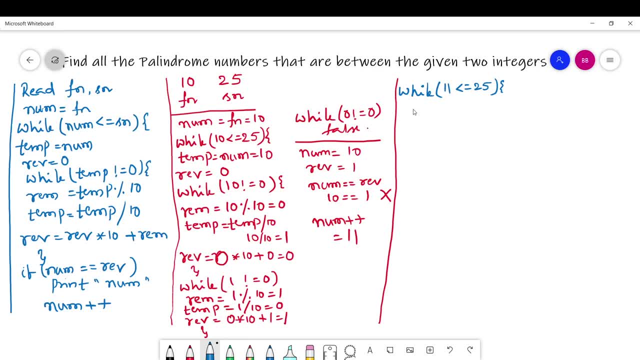 equals to 25. start temp is equals to number, that is 11. so 11 is assigned now as usual. reverse is once again initialized to 0 afterwards. now we will enter into the logic of finding the given number. is the present number, is palindrome or not? so 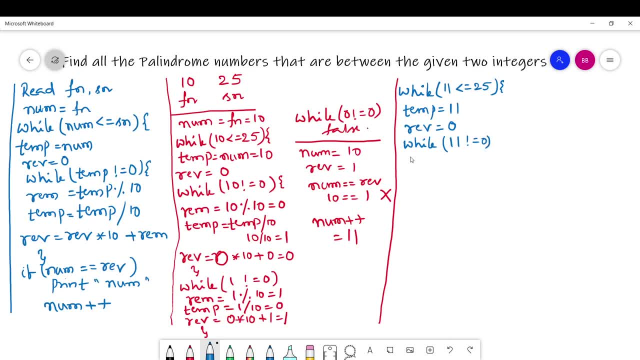 11 is not equal to 0. yes, it is true, because it is true. you're going to calculate the. the loop reminder is equals to 11, number, which is equals to 1, and thereafter we're going to calculate the new temp value, that is, 11 slash 10, which is equals to again 1. we. 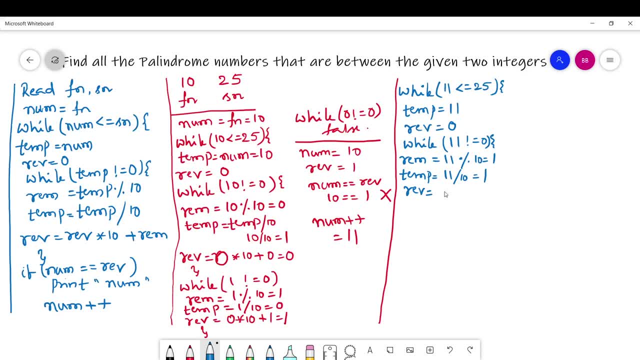 calculate the reverse value. reverse is reverse earlier. reverse is 0 into 10 plus rem- 한 갭InLanotve- misery-fine- and this 0 is 0 in to 3, Pls. rem плюс rem, that is 1. this is first iteration. let us see the second iteration, while second: 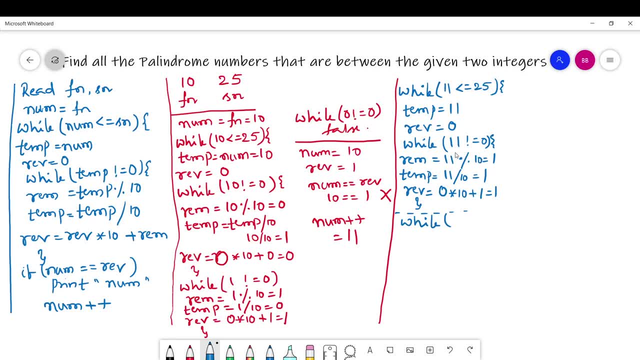 iteration is: while. what is the temp value? temp value is 1. 1 is not equal to 0, is not equal to 0, so it enters into the loop. then remainder is equals to 1 percent 10, which is 1. then temp is equals to 1 slash 10, that becomes 0. 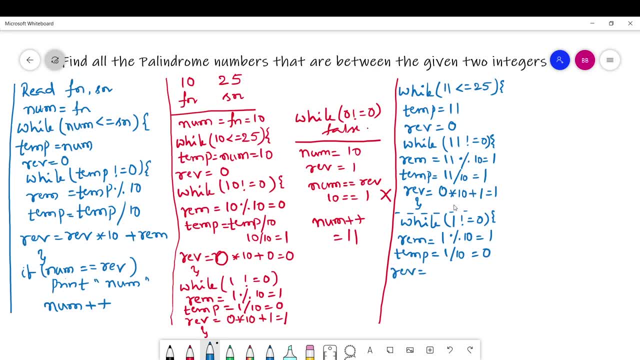 reverse. calculating the reverse reverse: earlier reverse is 1, 1 into 10, plus remainder is 1, which becomes 11. okay enough, let us see whether we will be able to continue the 1 loop or not. so while what is the new value of temp? temp value is 0, 0 is not.